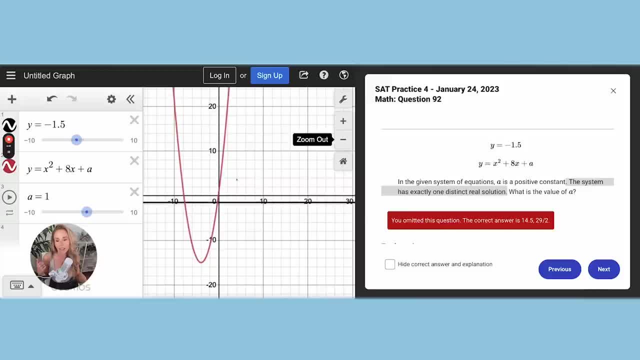 So if I have a quadratic- let me zoom out a little bit- and a line, I want the vertex to touch the line and that's it. You guys, take a look at this, Look at this answer. explanation from College Board. 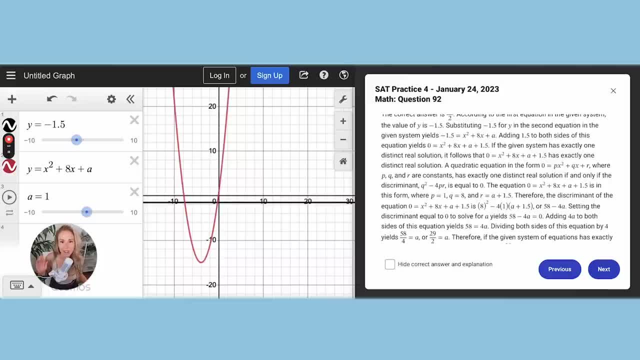 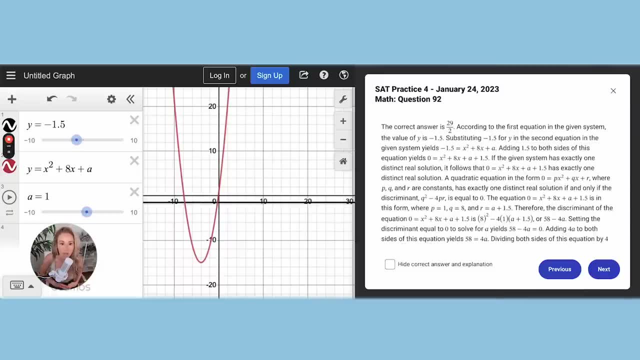 Like: are you kidding me? College Board, no, No, College Board- word Like this is just so ridiculous And, honestly, solving these graphically is way better than solving them algebraically. So if I want to find out what A is going to be, which is the Y, 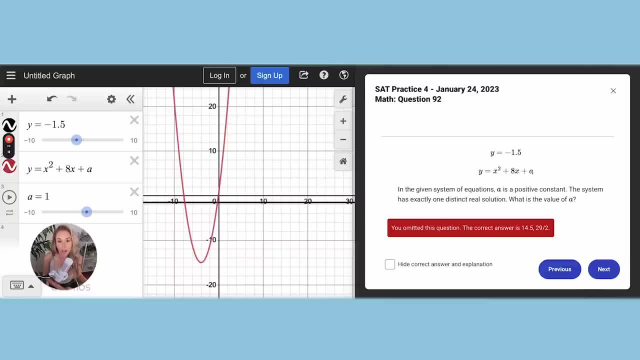 intercept of the quadratic when there's one solution, I'm going to move A around and I want to shift it up. I'm trying to get that vertex to touch the line. You see how I'm not quite there yet. What I have to do is I have to change the range of A, because right now it's going from. 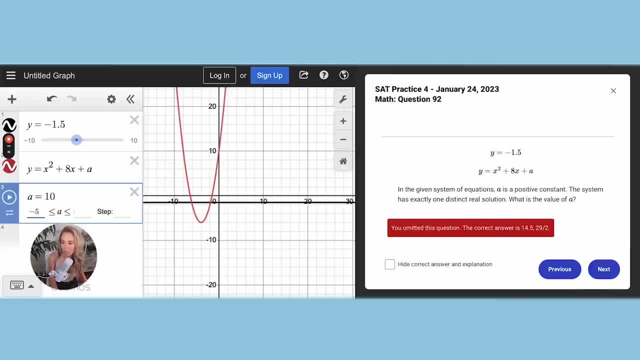 negative 10 to 10.. So let me just make it from like negative five to 50.. Okay, And what I'm going to do too, is I'm going to add in a step of 0.1, because I want to be able to move it incrementally. 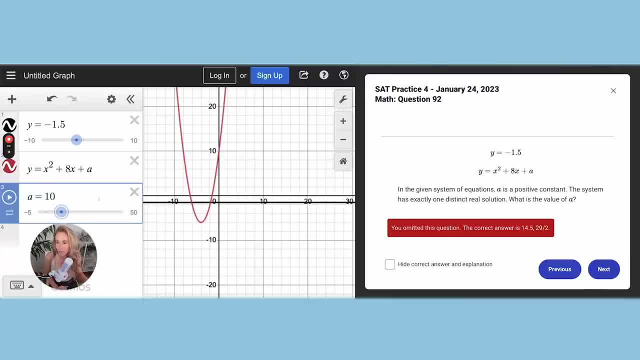 just in case there's like a decimal or whatever. So we're going to try that out and I'm going to keep moving it and keep moving it Now, as you can see with my mouse when I scroll it to 14.5,. 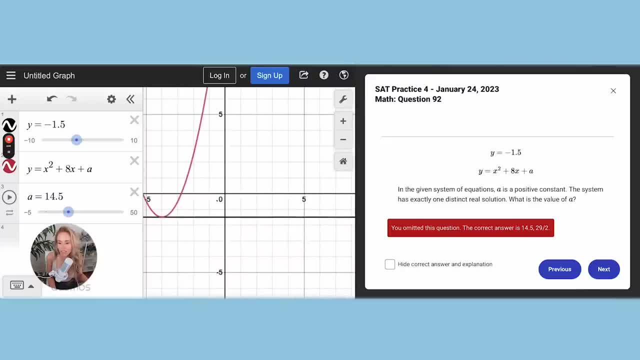 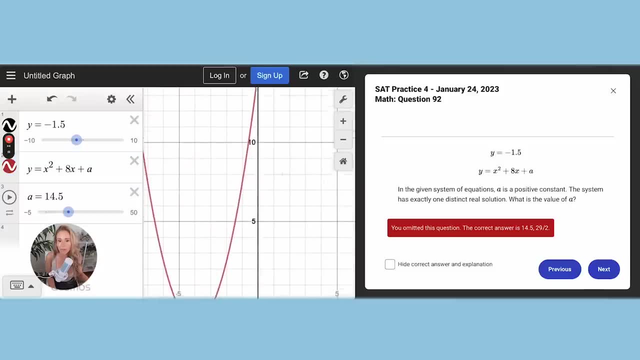 it's exactly. The vertex is exactly on the line, Do you guys see that? So that means A equals 14.5.. When that happens, as you can see, it crosses up here at 14.5.. And, as you can see, the correct answer. 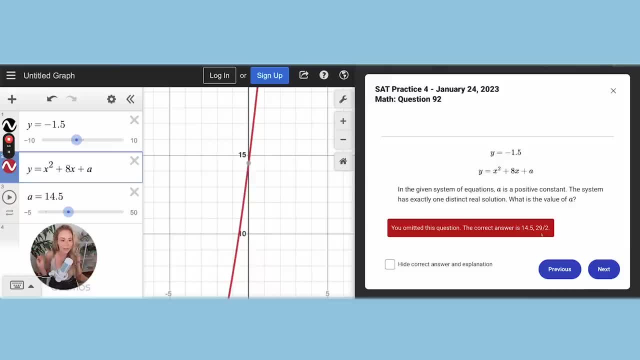 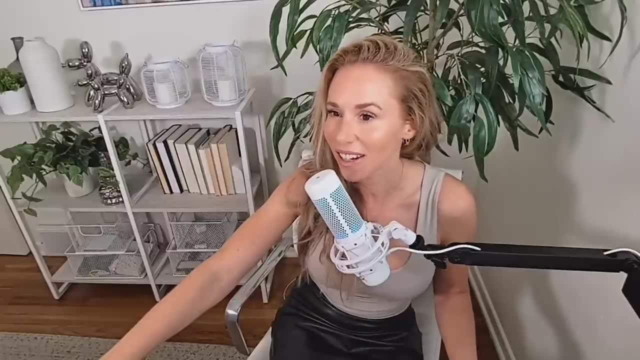 actually was 14.5.. Easy peasy, way better than doing all of that that College Board's telling you to do. All right, guys, I'm about to get to the next problem, But if you thought that that first example was helpful, make sure to hit the like button and subscribe to my channel. 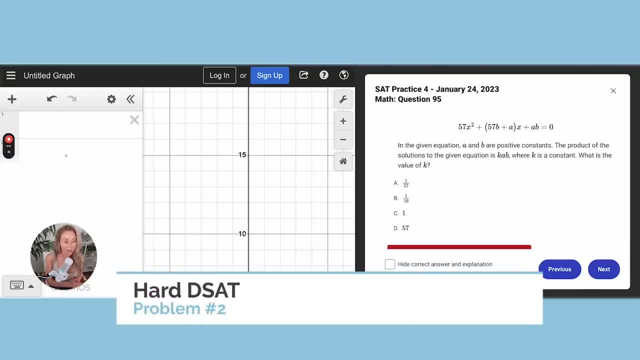 Hit the thumbs up button below. All right, this next one has a couple of constants in it, an A and a B, And it says the product of the solutions to the given equation is K times A times B, where K is a constant. Well, I already know that that's a quadratic, because 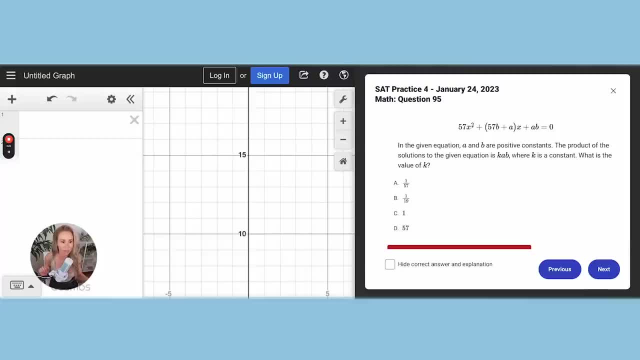 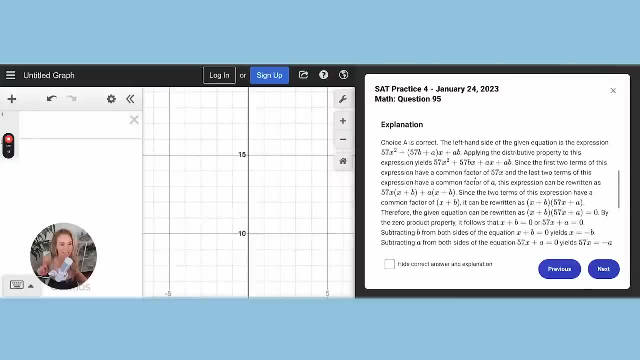 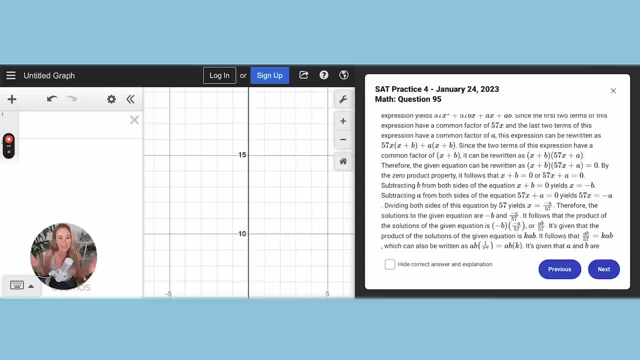 our highest exponent is squared, So there should be two solutions crossing the x-axis When we graph it. we're going to look for that, But look at this, you guys, look at this explanation. Have you guys been seeing this? I'm blue book. Like what is this? No, I would never, ever tell my students to do all of that. 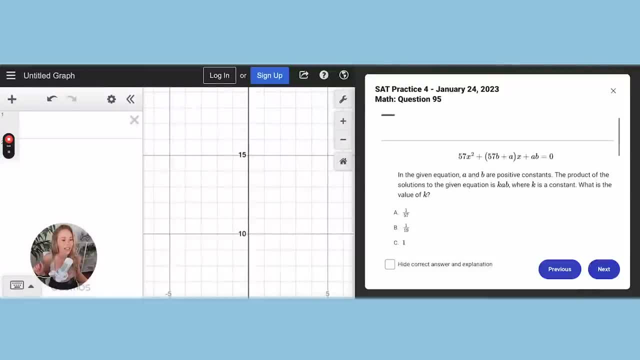 Do not do all of that, please. Okay, so here's what we're going to do. I'm going to type it back, the whole equation, into Desmos. Okay, I'm going to add a slider for both A and B. Now just make sure that you are doing what. 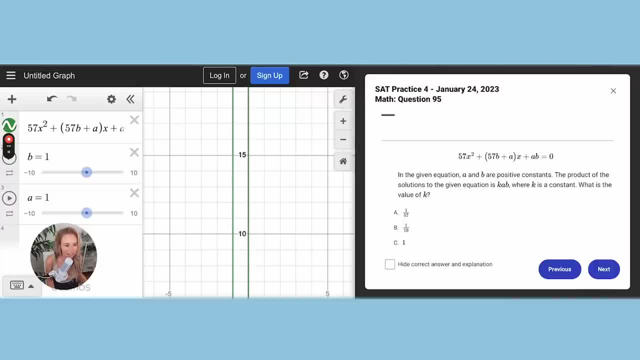 they're asking for. It says A and B are positive constants. Do you guys see that? So we just have to make sure that we keep A and B as positive numbers. Let me just zoom out just a little bit so you can see what's going on. 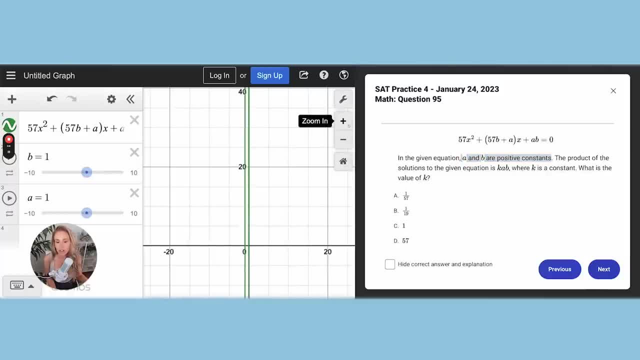 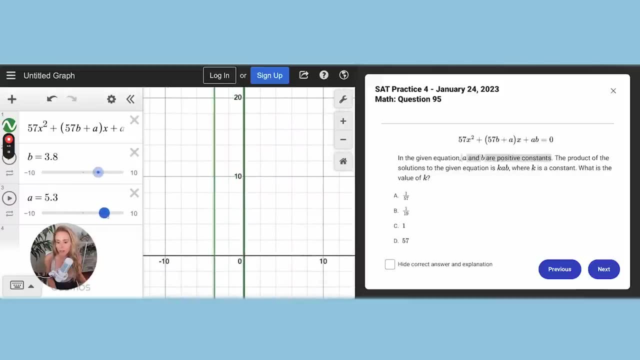 here. So right now we have a very narrow, narrow parabola. I could like mess with this and move these around and make it wider, But honestly, I actually like A and B to be one, because I just think it's easy, and I'll explain why. 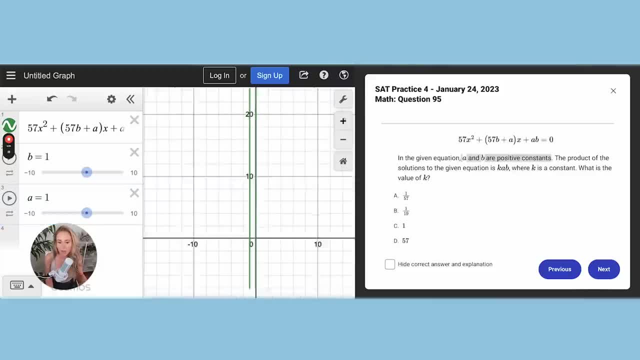 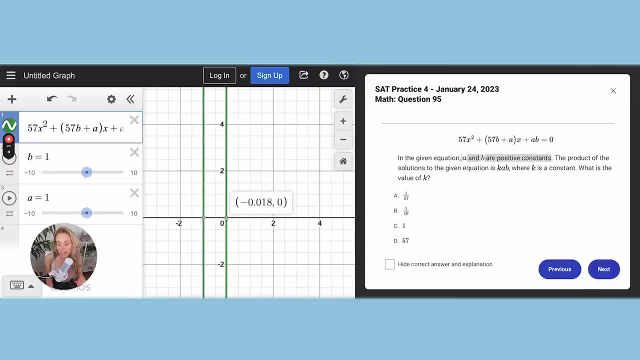 When A and B are one and I zoom in, I can see what the solutions are. So we've got a solution at negative one and at negative 0.018.. Okay, so that means negative one times negative 0.018.. 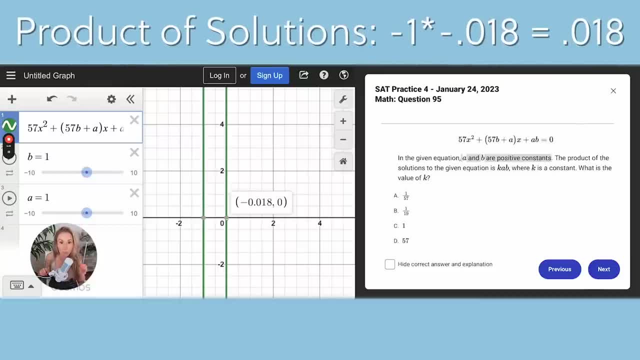 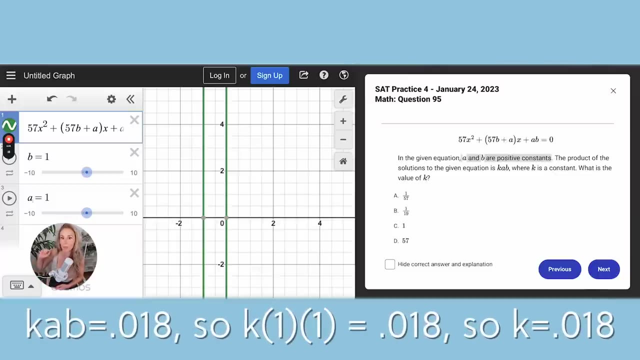 That's the product of the solution, So it would be a positive 0.018.. Okay, if A and B are one and then we multiply by K, that means K is going to have to be equal to 0.018, because one times one times 0.018 will get us the. 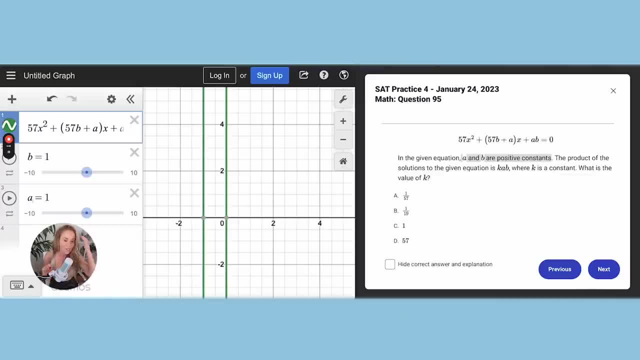 product of the solutions, which is 0.018.. So when you look at all the answer choices, they don't have it in decimal form. What you'll have to do is just in your calculator divide. So I could even pull up a calculator right now, or I could use Desmos too, but I'm in the graphene, So I just 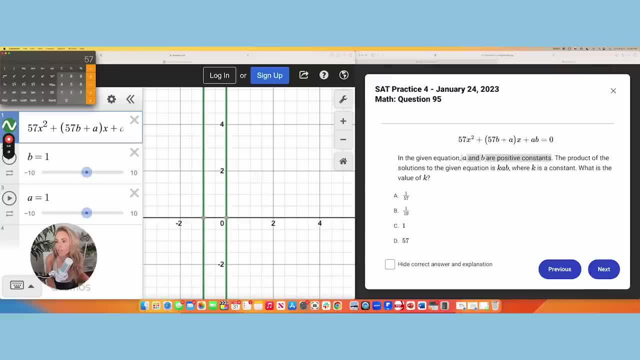 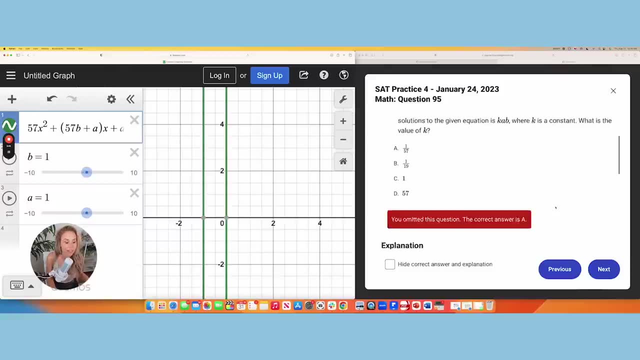 don't want to have to deal with that right now. So we've got one divided by 57.. And that rounds to 0.018.. So it's going to be A And, as you can see, the answer is A. So go, Desmos. 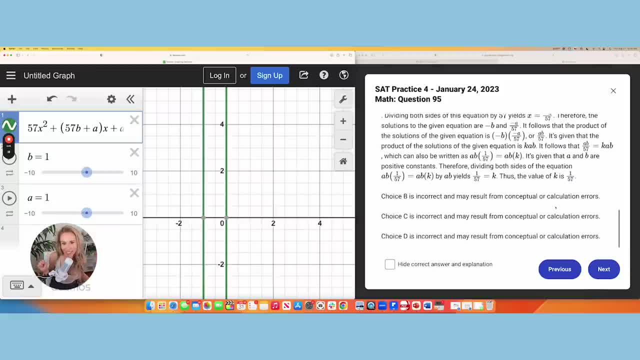 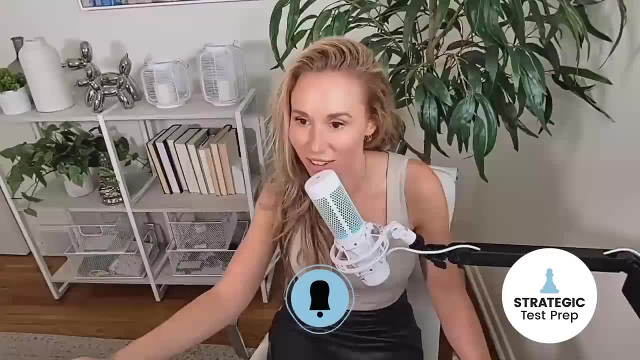 So much easier than doing all of that. Okay, let's go to the next one. All right guys? well, I'm looking for that next problem. If you haven't subscribed to my channel yet, make sure to hit the subscribe button below so you don't miss out on future content from me. to help you get ready for: 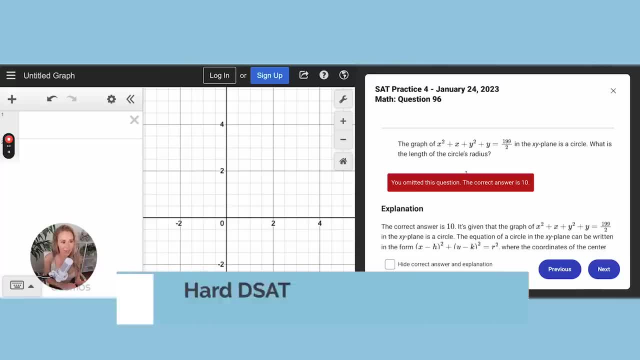 the DSAT. All right, so this next one is going to be A, So I'm going to go to. the next one is a circle equation, and they want the circle's radius. Yes, you can complete the square and do a whole bunch of stuff. It is equal to a nasty fraction. So that's going to be annoying, Look. 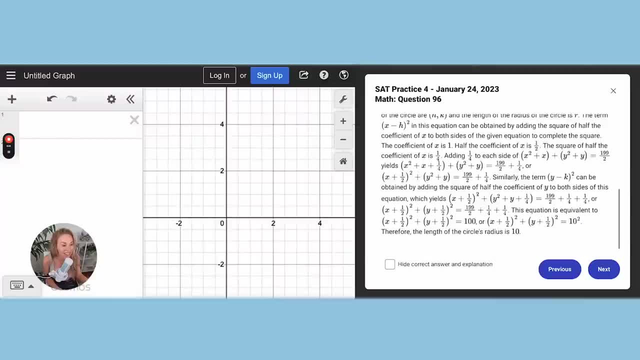 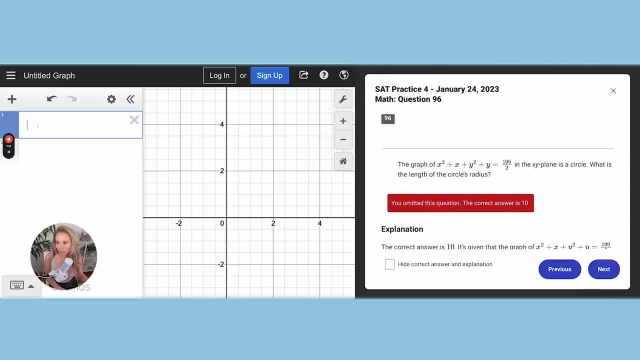 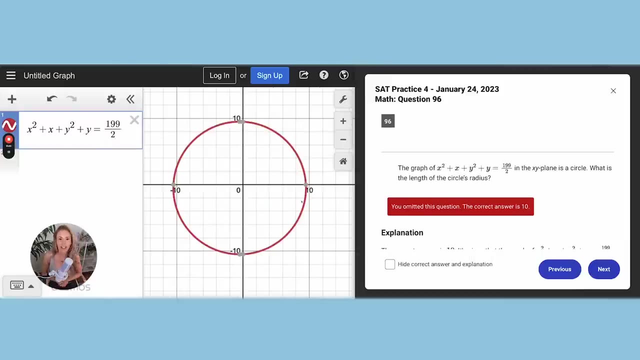 at their answer. explanation. you guys, No, Why, Why would you torture yourself? So I'm going to do the same thing as the others: I'm going to type this equation into Desmos. All right, guys. so we the circle graphed and, as you can see, it's a little off centered, so be very. 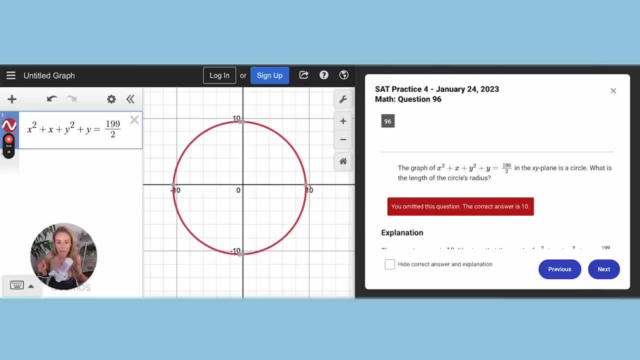 careful you can't assume the center is at zero and then just go: oh okay, so it's gonna be radius of nine point four, eight, seven. don't do that, because of course they're gonna try to throw you off and make it like a little bit different than. 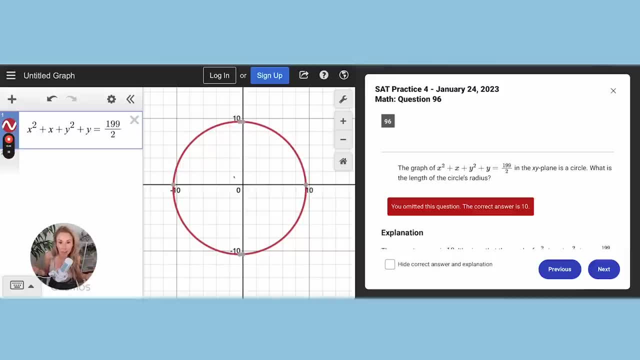 what you would assume. but what you can do is just find out how long the diameter is and divide it in half. so here's like an end point. I've got an endpoint at nine, point five, and then, if I go down here, I have another end point. 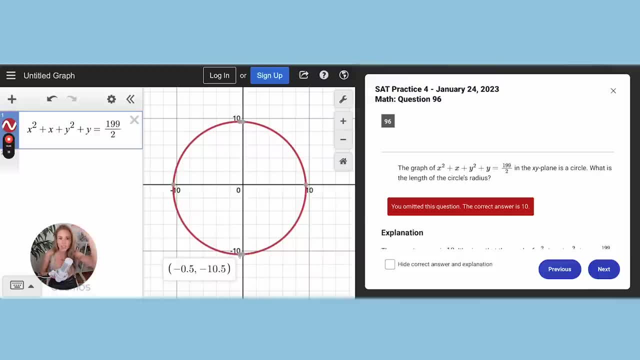 at negative ten point five. now, that's a distance of twenty units. divide that in half, your radius is ten and you're done, and, as you can see here, the correct answer is ten. so that's it, just a heads up. if you want more math problems to. 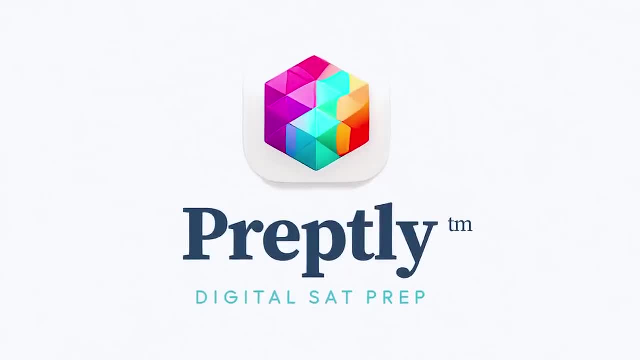 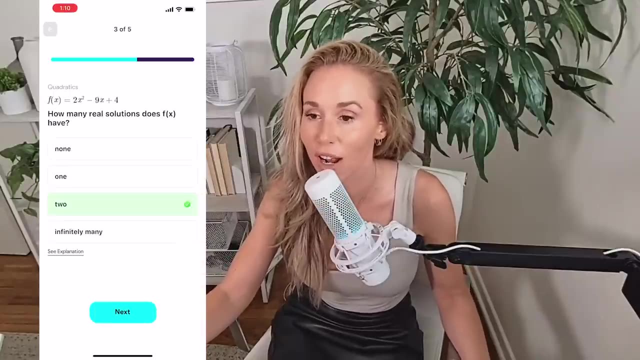 prep from for the D set. make sure to download properly in the App Store or in Google Play today, so that you can keep prepping for the math with an array of additional problems that are just like those on Blue Book. okay, so this last one is super. 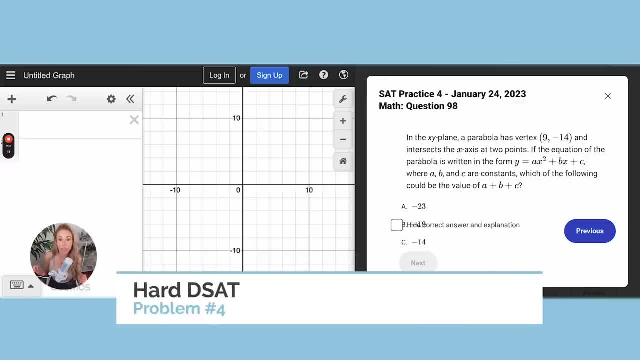 tricky and involves a little logical reasoning, but you can still use Desmos to help you get the answer. so it says: in the XY plane, a parabola has vertex nine negative fourteen and intersects the x-axis at two points. okay, if the vertex is at nine negative fourteen, I'm gonna go ahead and type in an equation in: 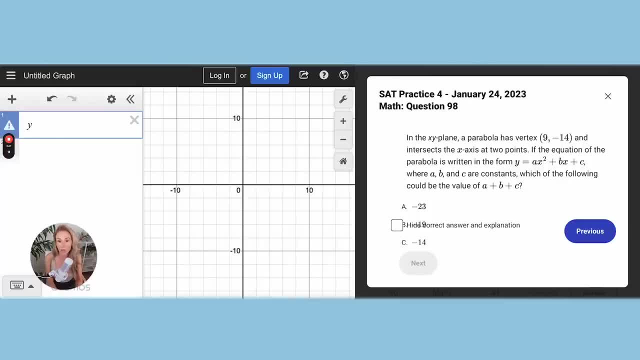 vertex form. so the only thing we don't know is the a. we don't know if it's flipping up or down. we don't know if it's wide or narrow, so I'm just gonna leave it as an a and put a slider in now that. 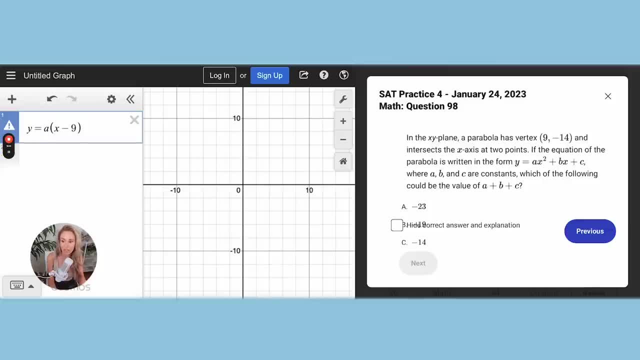 should be an X minus nine, because the vertex x-coordinate changes the sign, so if it's a nine, then it should be a minus nine, in the parentheses, and the y coordinate stays the same at negative fourteen. let's add in a slider and we're gonna start to mess with this now. it said that: 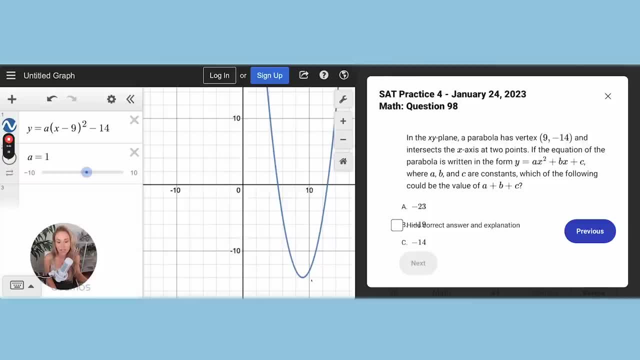 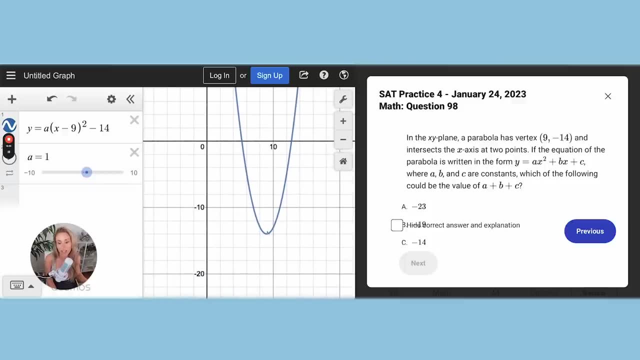 it intersects the x-axis at two points. so, as you guys can see, our vertex is down here. so if our vertex is in quadrant four and it's like in this negative y area, we have to have an a that's positive, because this parabola has to be able to flip up to have two solutions crossing the x-axis. okay, so we 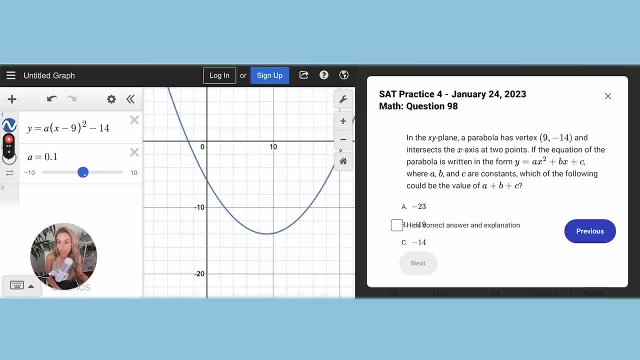 know a needs to be positive. if we mess with this, look at once you get past positive point one up. now it's flat, and now it goes down, and now it's not crossing anymore. so a's got to be a positive number. now we know B in the quadratic, that's. that's a left and right shift. so since 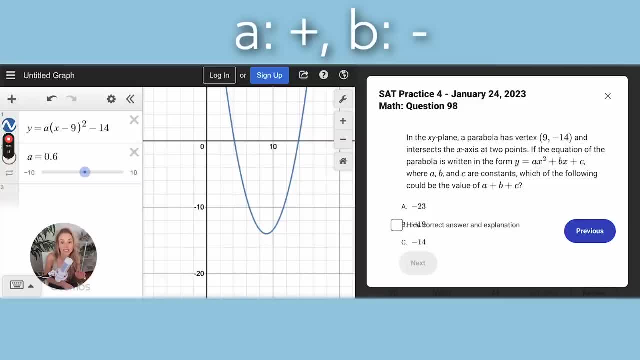 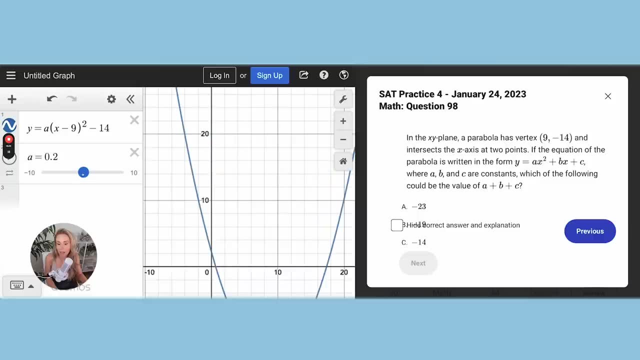 this parabola is shifted to the right. that means B is negative and it looks like when we mess with this, we mess with the a for the most part- check that out- C is positive. C is where the y-intercept is. there's only one time where C is. 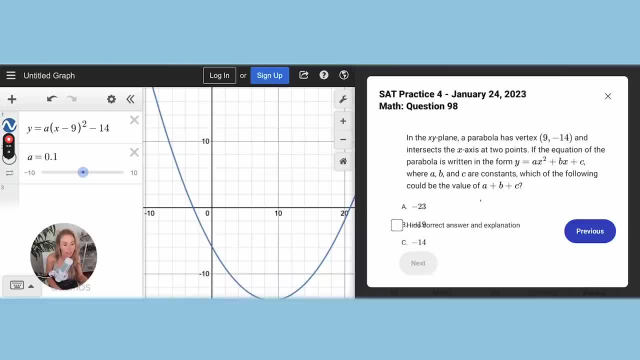 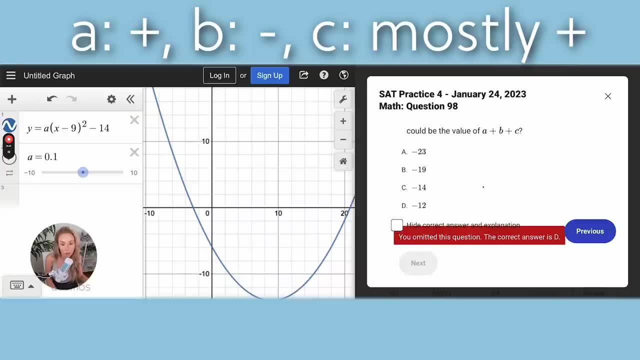 negative, so a has to be a positive and a has to be a negative, so a has to be a positive. C, for the most part, is positive. the only one that's negative is B. so use your logical reasoning. if a and C are positive and B is negative, you've